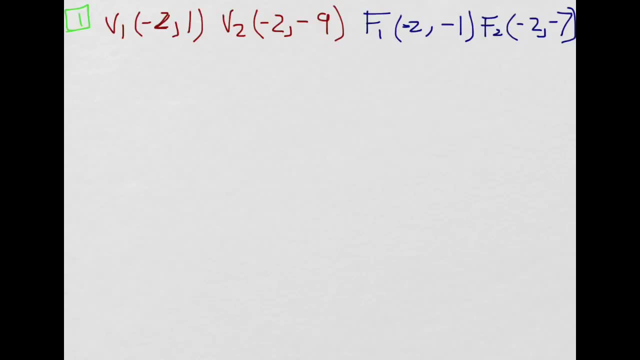 to do everything. So let's go ahead and get started. We are given the two vertices and two foci of a conic section, so it's either an elliptic or a vertical, And we're going to go ahead and plot the two vertices and the two foci. So let's think about what we know already. 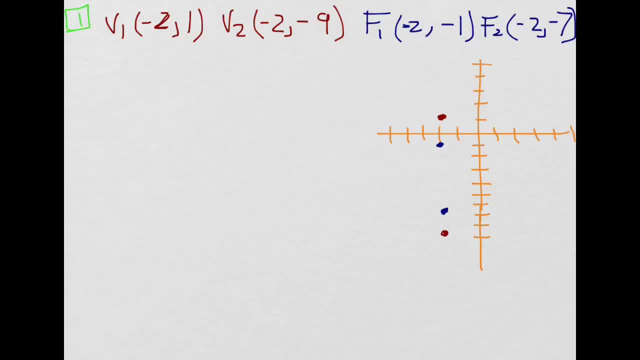 First off, we know this has to be a conic section, So we're going to go ahead and plot the two vertices and the two foci. So let's think about what we know already. First off, we know this has to be a vertical conic section because all the vertices and foci are lined up vertically. Past. 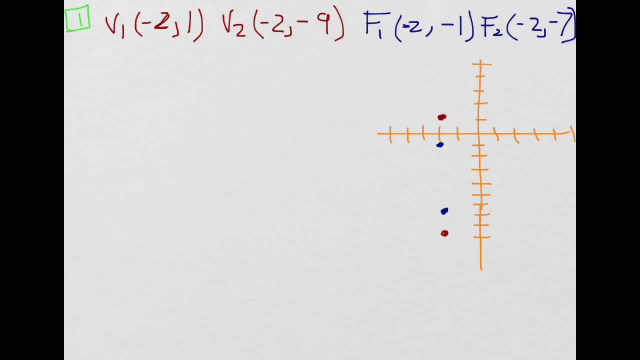 that we know that this has to be an ellipse, since the foci are on the inside. And if we want, now we can go through and we can find the center of the ellipse by going halfway between our foci. equivalently, Also, we could find it by going halfway between the vertices. Same exact 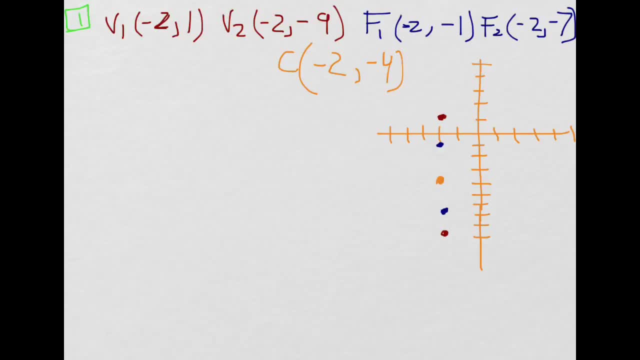 thing. So let's go ahead and identify that. So, for example, if you look at your two foci, one has a y value of negative one, the other has a y value of negative seven, a distance of six between those two points. So go three down from the top foci or three up from the bottom foci and end up at the. 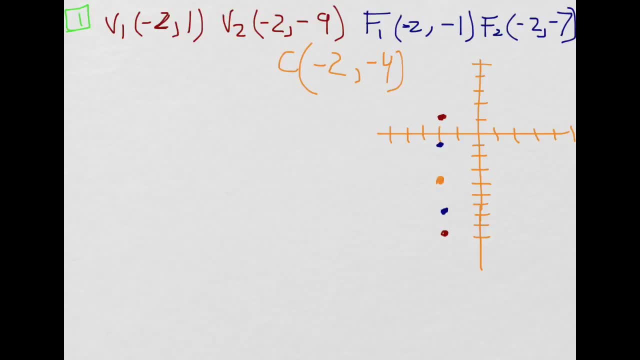 point, negative two, comma, negative four for the center of this ellipse. That is useful to us because now we can figure out our a value center of the ellipse, So we can go through and we can find the center to the vertex and also our c value which is the center to the focus. So I figured 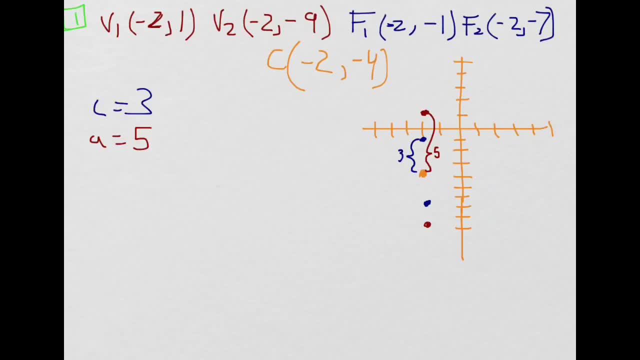 out going either direction, but let's go ahead and find those values. So c, the distance from the center to the foci is three. And if you can't remember a, b and c, what's what? remember that c is the center to the foci, because the foci or focus has the c in it. So that's c. That's how I. 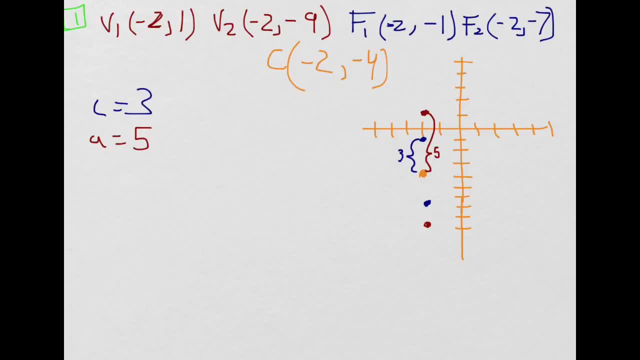 did it anyways. And then you know, a is always going to be from your center to your vertex. So in this case that is five. And remember, we have the equation that is almost like the Pythagorean theorem. It says c squared equals a squared minus b squared. So we can find the value of b. 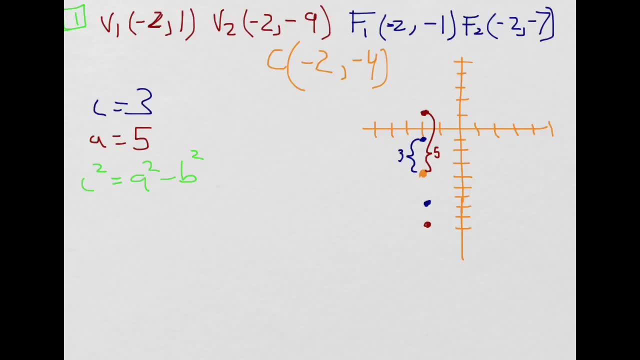 half of our semi-minor axis. If we substitute our values in, we get nine by squaring three equals 25 by squaring five minus b squared. So if we rearrange that, we get b squared equals 25 minus nine. So b squared equals 16, and hence b equals four. So now we can finish. 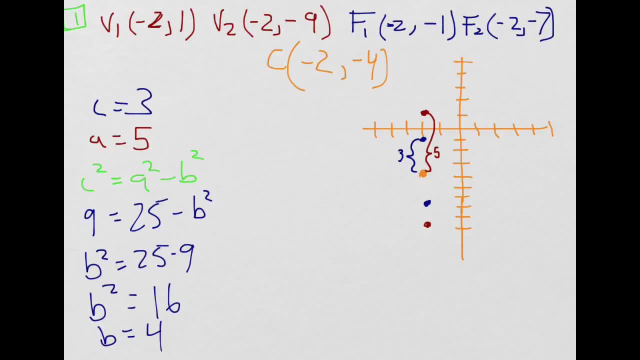 up this sketch because we know the half of the semi-minor axis is four, which means go to your center and go four to the right and four to the left to figure out those co-vertices. Let's go one, two, three, four- We're going to end up there- And one, two, three, four in the other direction- We're going to end up about there And we can sketch in this. 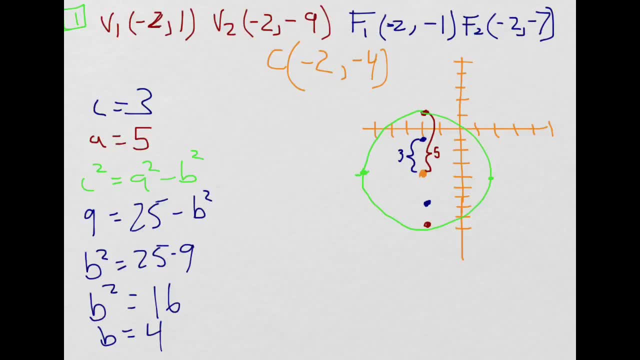 ellipse. That's not the best sketch I've ever done. Yours should look better because it's harder to do this on the iPad than it is to do it by hand. So at this point we know where our foci are. We. 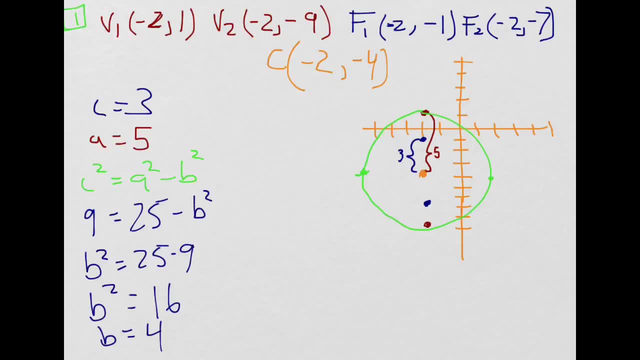 know where our vertices are. We know our values for a, b and c, So all that's left to do is write these two equations in rectangular form and also in parametric form. So, remember, we are dealing with the equation of a vertical ellipse, And so 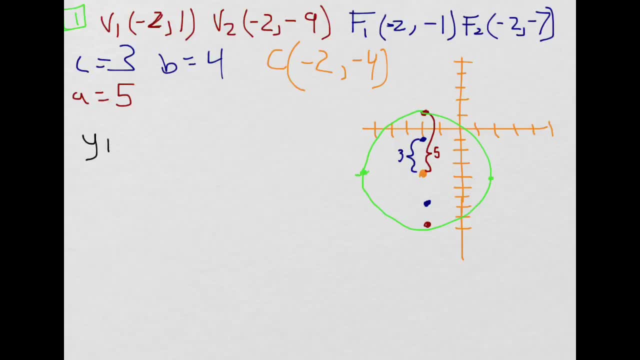 that is going to be y, already messed up. y minus k, quantity squared over a squared, And a is with y because it's vertical. Remember a has to be bigger than b. So y minus k squared over a squared plus x minus h, quantity squared. 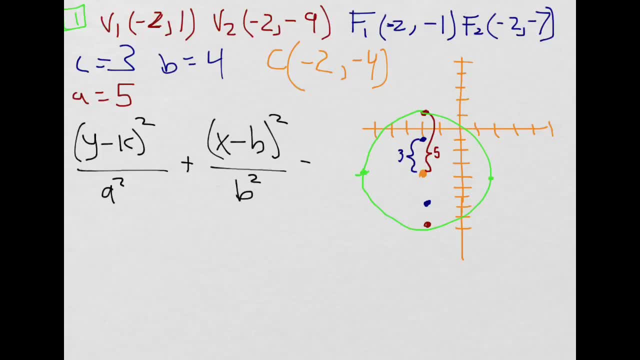 over b squared. b squared equals 1.. So substitute all of your values in y and since our center is down at what is that? 1,, 2,, 3,, 4, it's at a y value of negative 4.. We're going to 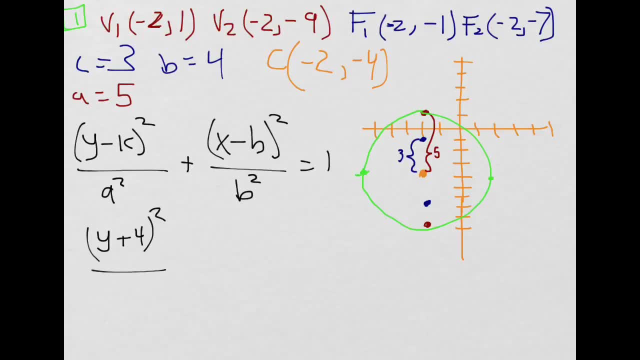 get y plus 4 squared over. a squared a is 5.. So you can just write it as 5 squared. I'm actually good with that. It looks better, I think, because you know what a is right away. So, plus parentheses, x plus 2 squared. because again we want to move that to the left, 2,. 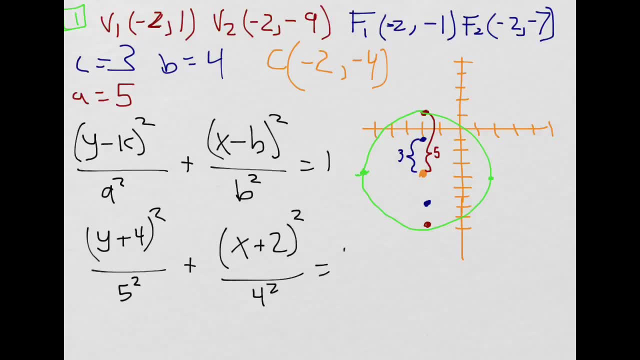 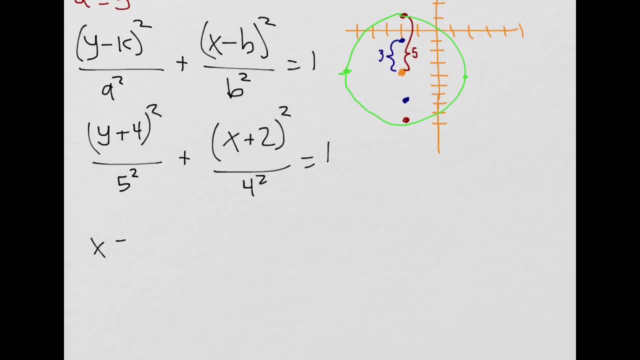 over b squared, b is 4.. So over 4 squared equals 1.. And now if we want to write this in parametric mode: x equals, y equals. Remember the Pythagorean identity. We can use that to get our parameterization quite clearly. 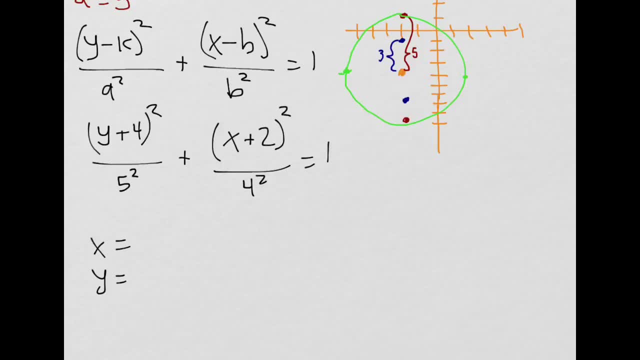 Thank you. quickly, it's going to be: x equals b times the cosine of t or theta, whatever you want to write, plus, oops, sorry, minus 2.. Okay, I'm just here's what I want to do: b equals. 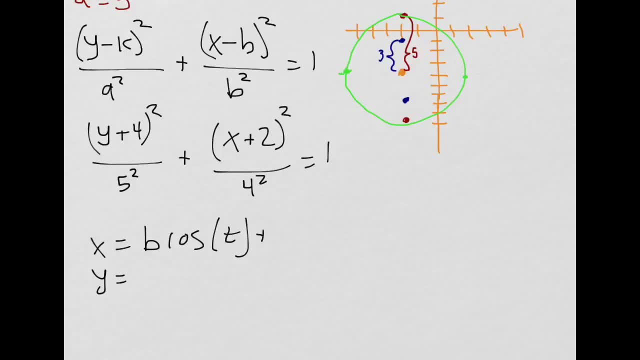 cosine t plus h and y equals a sine t plus k. Those are going to be our parameterizations. So when we substitute our values in, we're going to get x and notice b is with x and a is with y, again because it's a vertical ellipse. So now substitute our values in. 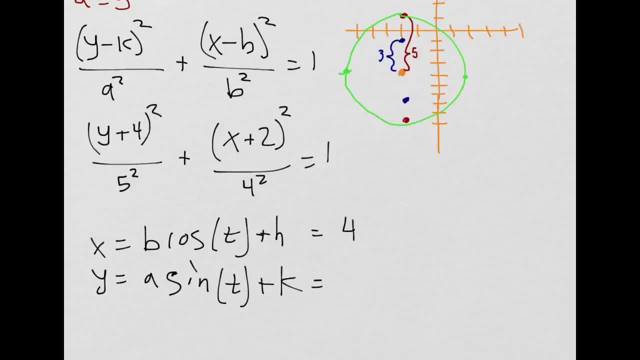 b is 4, so x equals 4.. 4 times the cosine of t, and since our h value is negative, 2, we get minus 2.. Notice in rectangular form the number is opposite that positive 2, even though we want the value negative. 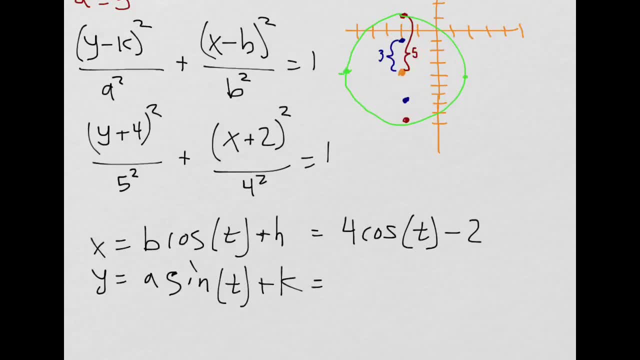 2, but in parametric mode it actually is that h value. And then finally we're going to get 5 sine of t and our y value is negative 2.. So again, it's going to be minus 4.. Now the starting point of this parameterization. 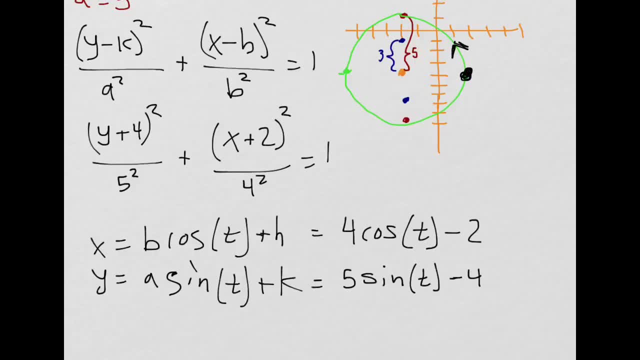 is going to be right there and our orientation is going to be counterclockwise. Remember, because x is with cosine and y is with sine. If you flipped it, if you had 4 sine t minus 2 for x and 5 cosine t minus 4 for y, our starting point would be: